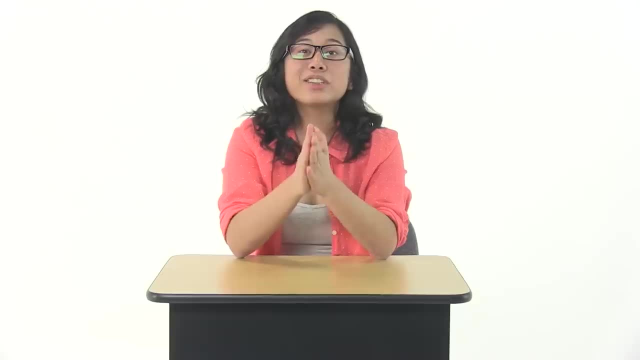 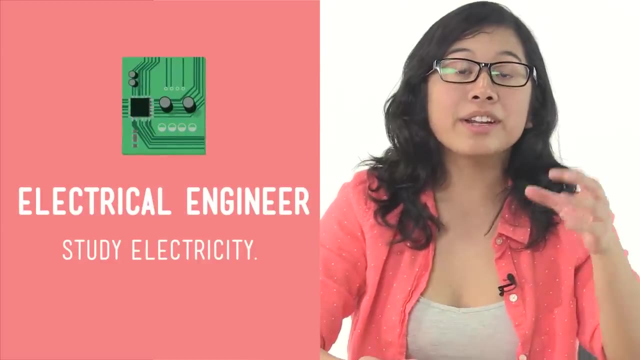 nuclear and software engineers, and the list goes on. Let's talk about what some of the other types of engineers do. First up, electrical engineers. Electrical engineers study electricity. They design electrical systems like circuits and computer chips. Think of an electrical object that you use pretty regularly. 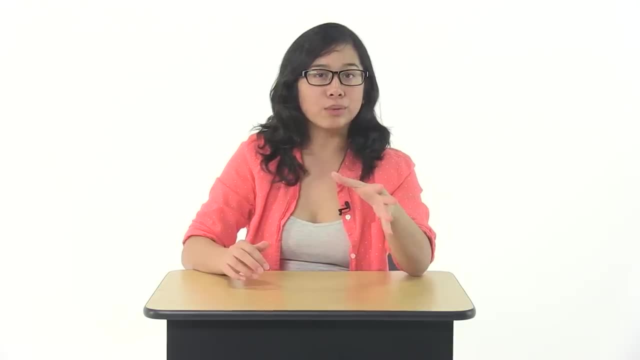 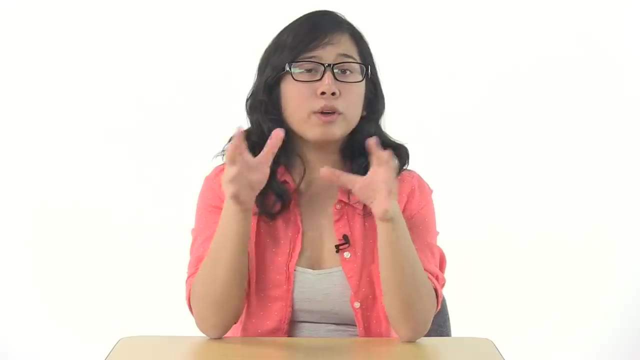 How about your microwave? What problem was the microwave? a solution to Cold food, right? Yes, You need an electrical engineer to thank for the ability to reheat that leftover pizza you just had for lunch. But while you might not have heard of Joseph Strauss or Percy Spencer, the engineers responsible, 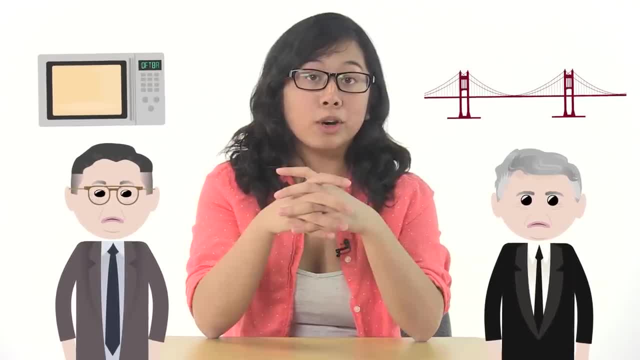 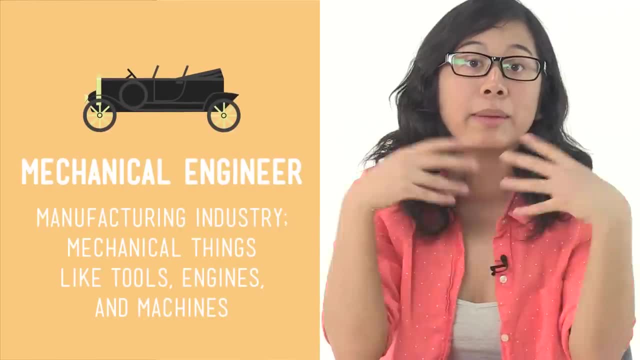 for the Golden Gate Bridge and the microwave respectively. you've probably heard of Henry Ford, As in Ford cars, Henry Ford was a mechanical engineer or someone working in the manufacturing industry making mechanical things like tools, engines and machines, Machines like cars. Ford didn't invent the automobile, but his Ford Motor Company made a lot of them. His Model T car was famous for being affordable for plenty of Americans. Ford saw that lots of people who wanted to drive cars just couldn't because they couldn't. 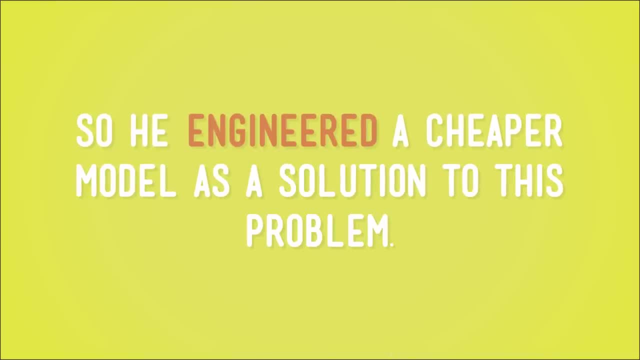 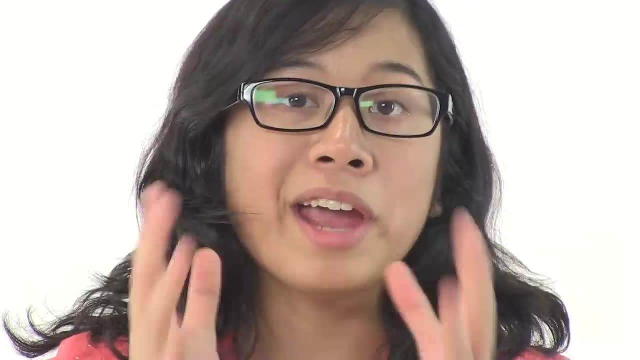 afford the pricey vehicles that were for sale, So he engineered a cheaper model as a solution to this problem. His fellow engineers started to do the same and now, well, cars are everywhere. Henry Ford's not the only big-name engineer. A famous engineer around today is Marissa Mayer. 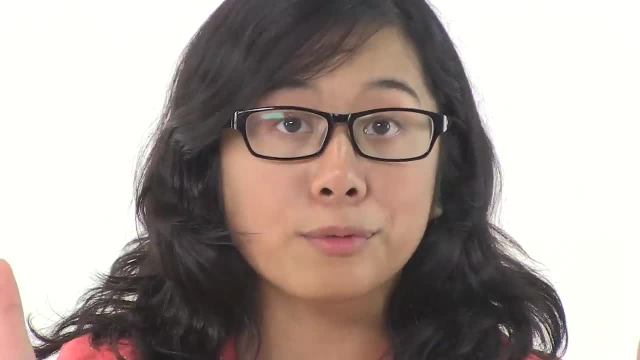 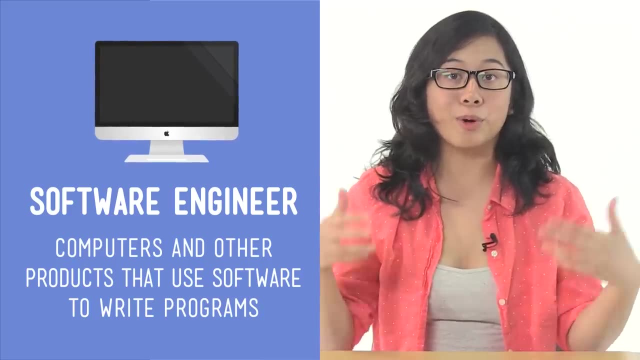 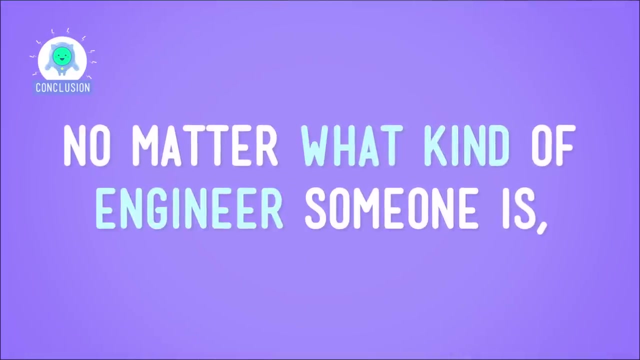 Mayer is the president of the internet company Yahoo and is also a software engineer. Software engineers work on computers And other products that use software to write programs to make them faster and able to do more things. No matter what kind of engineer someone is, their job at its most basic level is problem. 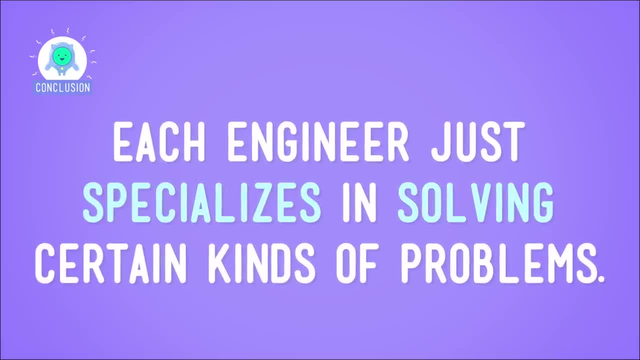 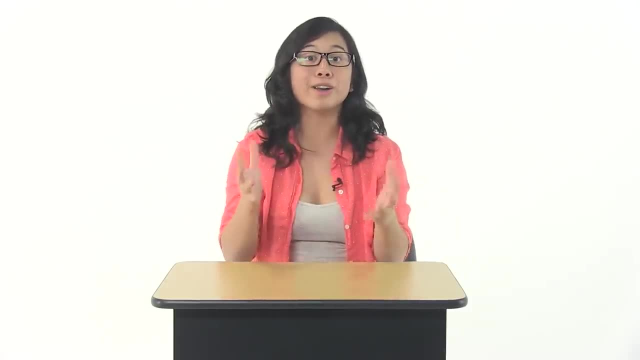 solving. Each engineer just specializes in solving certain kinds of problems. While it might seem like there are too many types of engineers to keep track of, just wait fifteen years, or fifty, or one hundred, because we'll probably have a ton of different. 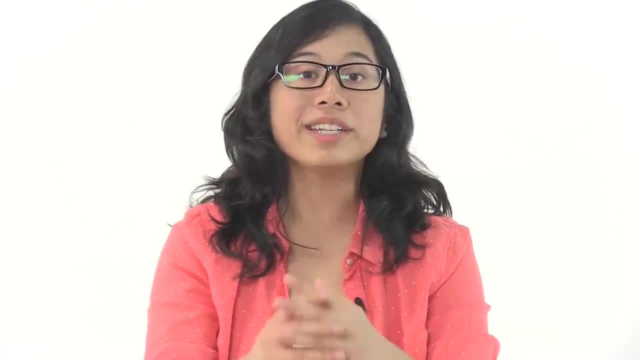 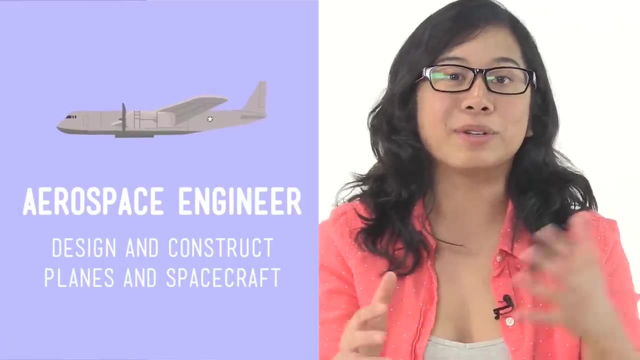 types to add to the list. Think about it: Over a hundred years ago we didn't have jobs in fields like aerospace engineering, where people design and construct planes and spacecraft. We didn't have planes like we do today or need spaceships, so we didn't need people. 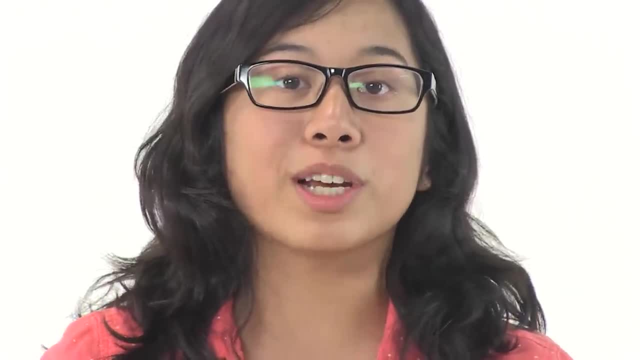 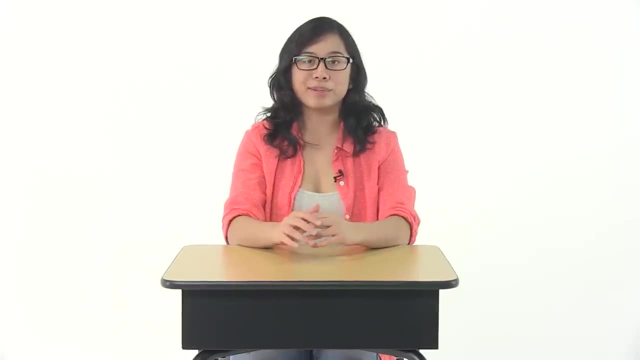 to engineer them. Who knows what machines or tools or everyday objects we'll have in the year 3015?? Personally, I'm hoping for underwater cities, But whatever these things are, we'll need engineers to make them. So what do you say?